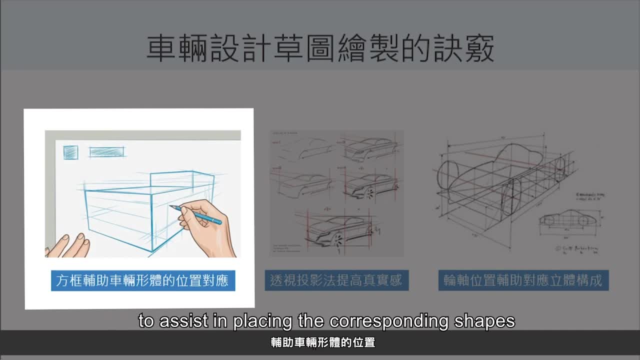 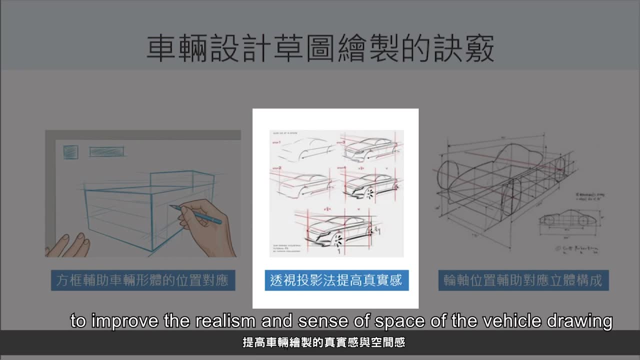 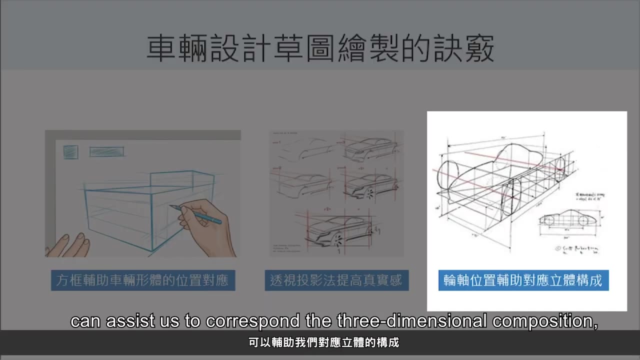 For example, We can draw draw some rectangular frames to assist in placing the corresponding shapes of the vehicle within this cube. At the same time, we can use perspective projection to improve the realism and sense of space of the vehicle. drawing The position of the vehicle axles can assist us to correspond the three-dimensional composition. 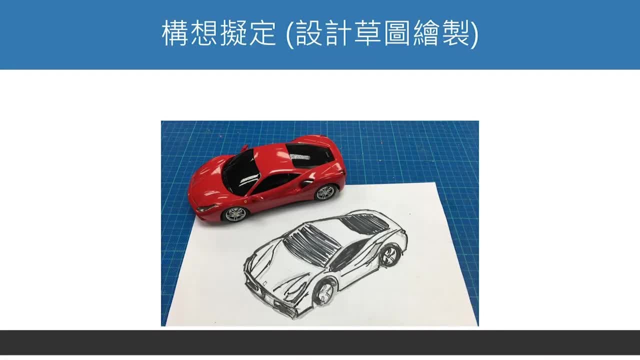 so that the three-dimensional sense of space of the vehicle is more real. Here we arrange an activity for concept design planning and sketch drawing. After watching the teacher's demonstration you can turn your concept ideas about the compressed air racing car into concrete concept design sketches and prepare several design. 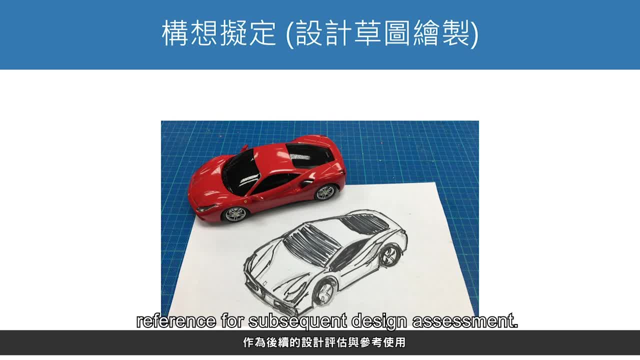 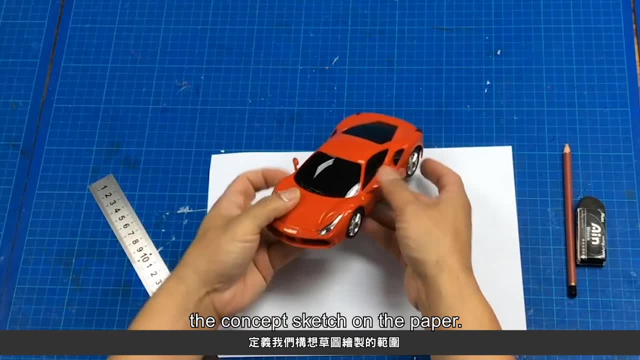 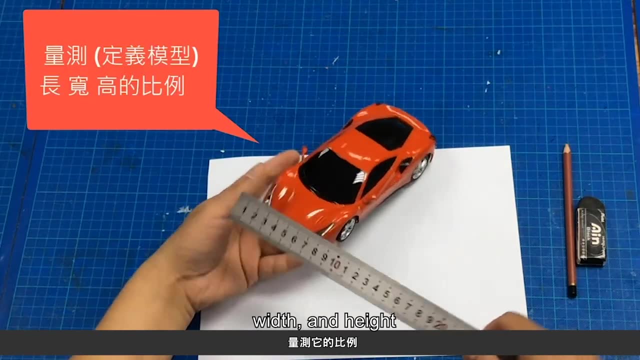 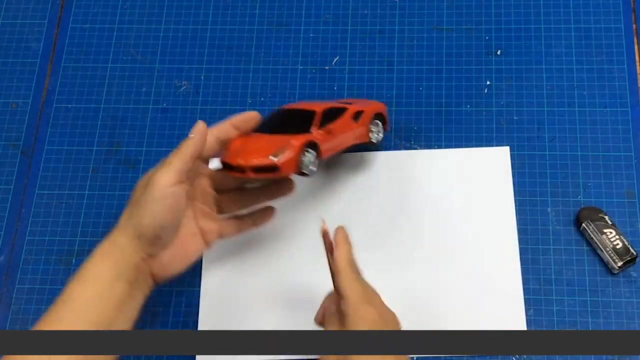 schemes as reference for subsequent design assessment. First, let's define the drawing area of the concept sketch on the paper. We measure the scale of the model by its length, width and height And draw a three-dimensional cube corresponding the position of the model on our paper. 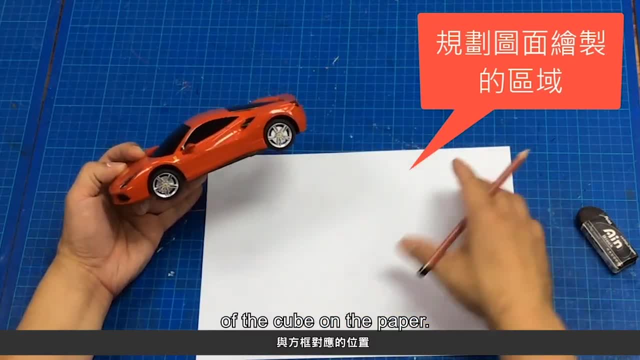 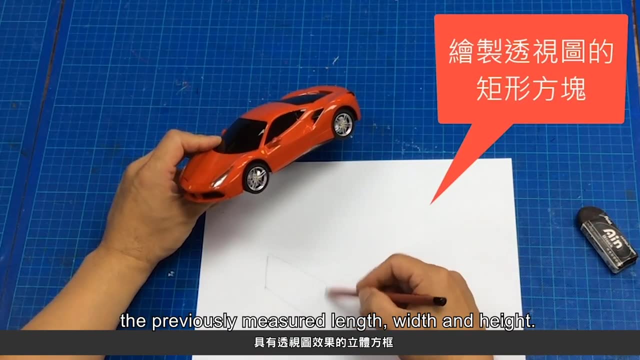 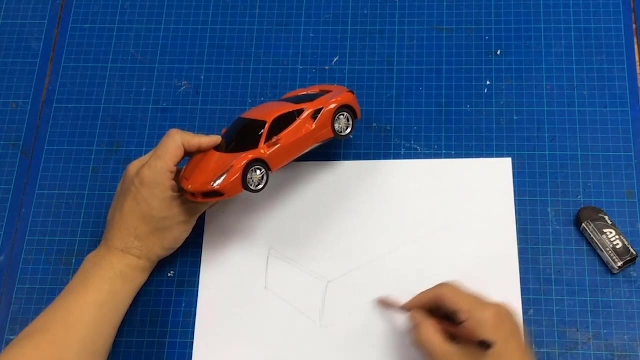 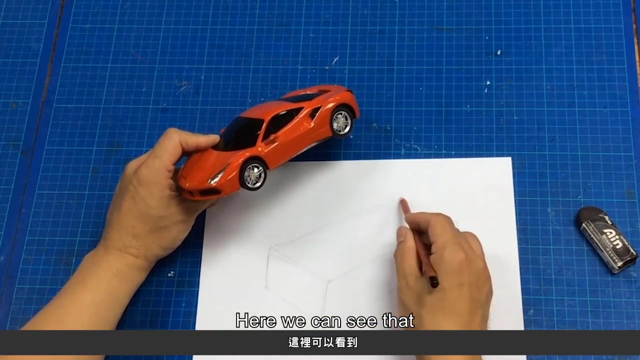 Before drawing, we first plan the corresponding position of the cube on the paper. We draw a three-dimensional cube with perspective effect according to the previously measured length, width and height. Here we can see that there is a vanishing point by extending the lines in the length. 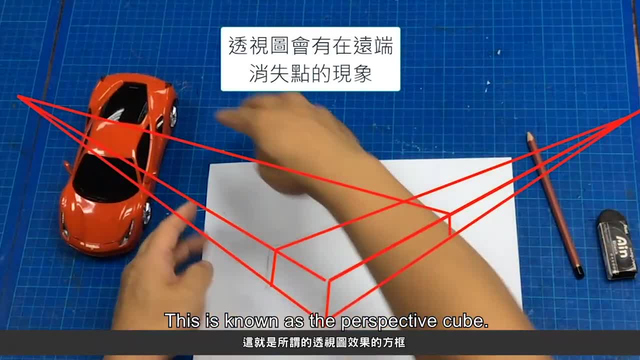 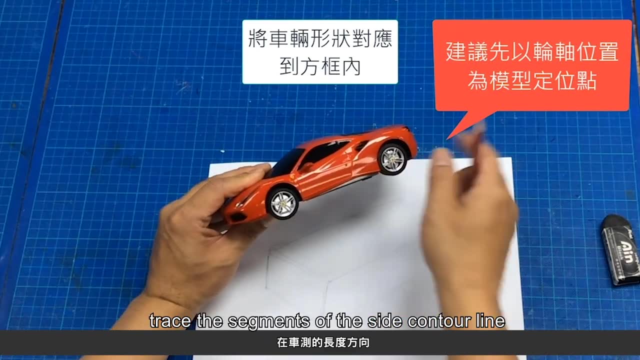 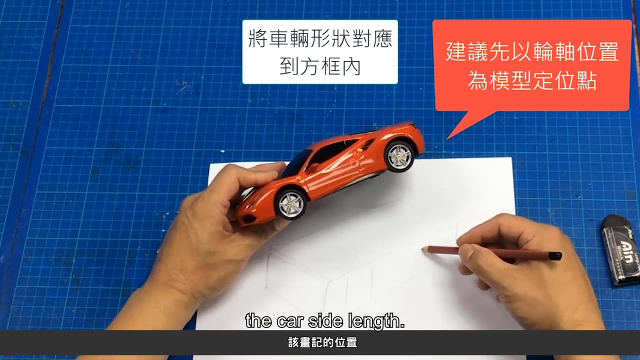 direction. This also happens in the width direction. This is known as the perspective cube. Next, we use the corresponding position of the wheel axle to trace the segments of the side contour line in the direction of the car side length When drawing the round wheels. 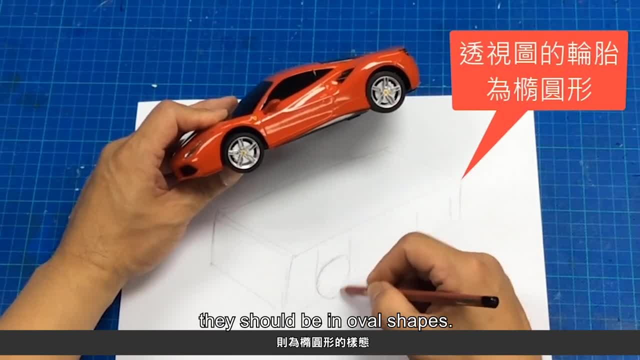 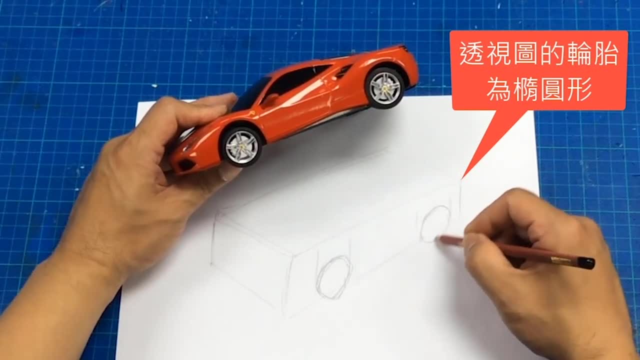 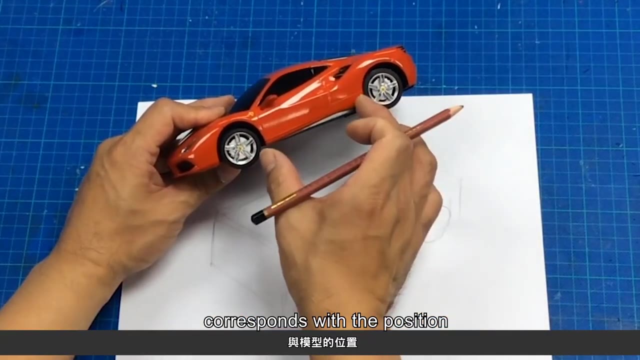 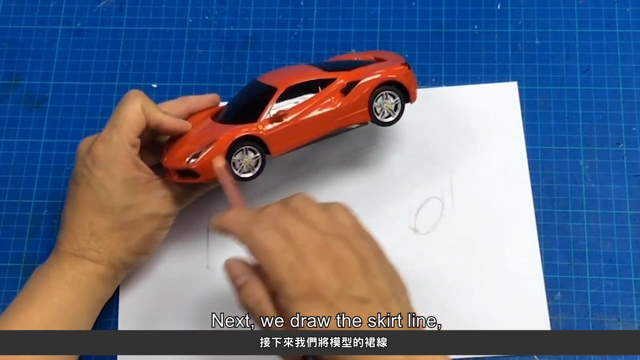 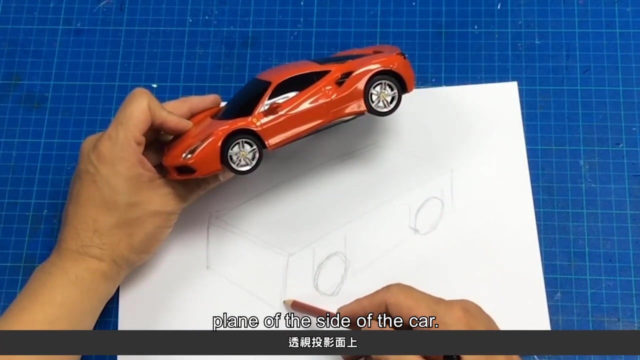 On the perspective drawing. they should be in oval shapes. Check if the tires on the side of the car corresponds with the position of the model. Next we draw the skirt line, waist line and shoulder line of the model on the perspective projection plane on the side of the car. 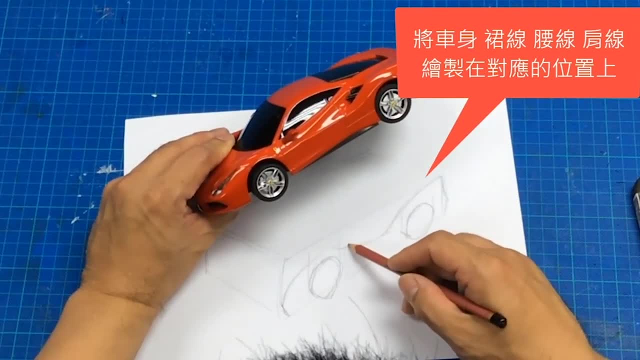 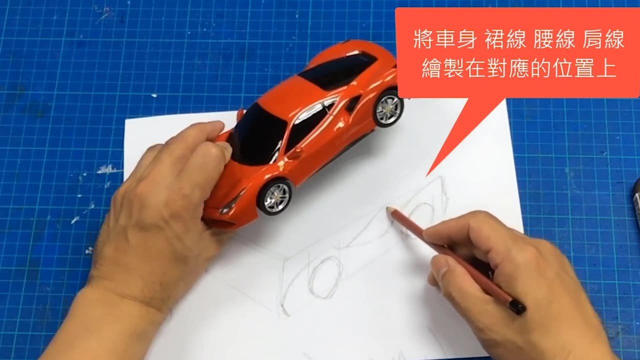 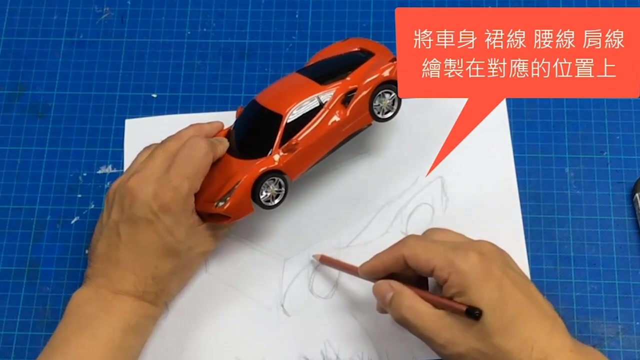 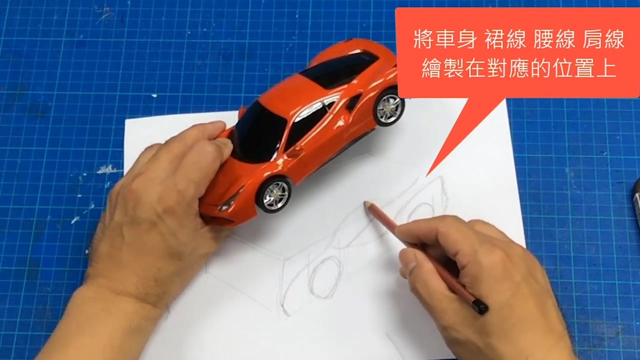 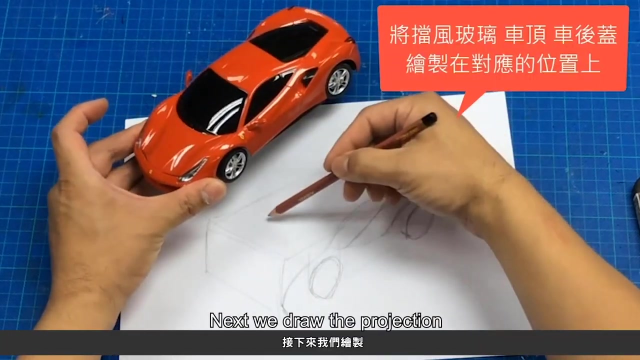 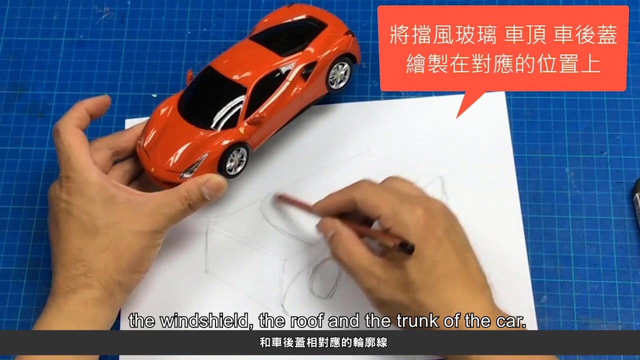 Then we draw the body line on the perspective projection plane with dimensions of 40 inches per inch, which can be calculated by the chromatic direction. To do this we will need to set three wheels, with the sometimes Fred. Next, we draw the projection plane of the top view of the vehicle, which are lines corresponding to the windshield, the roof and the trunk of the car. 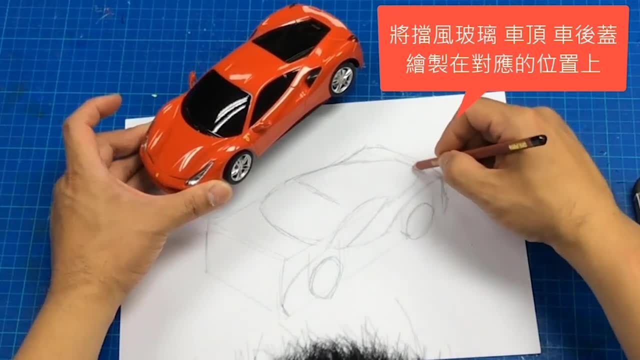 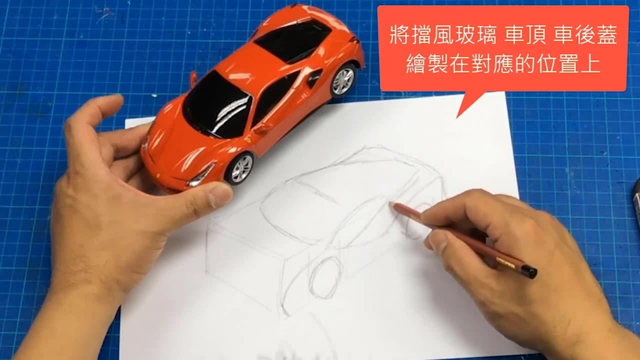 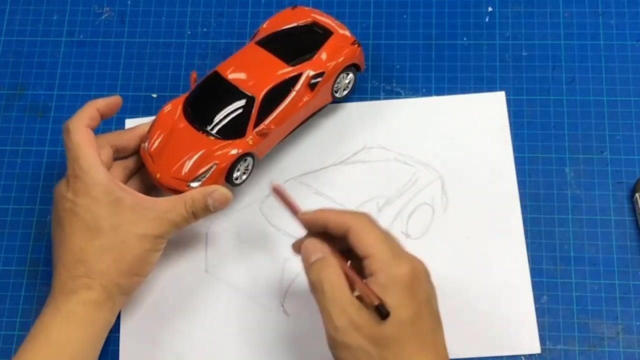 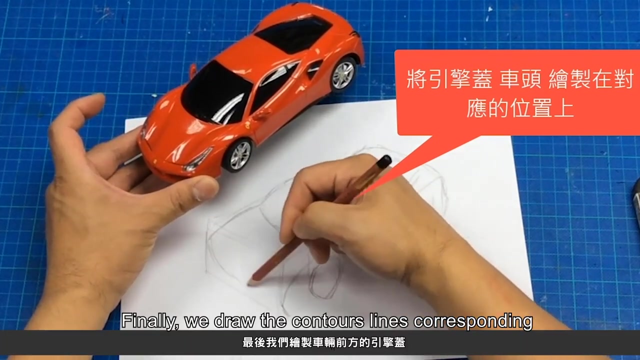 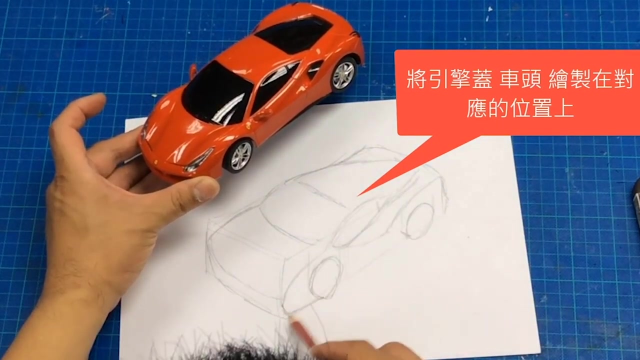 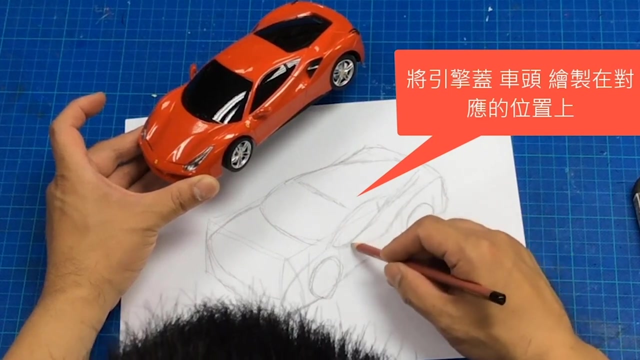 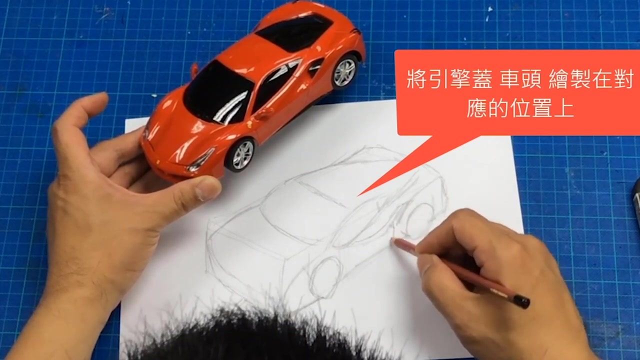 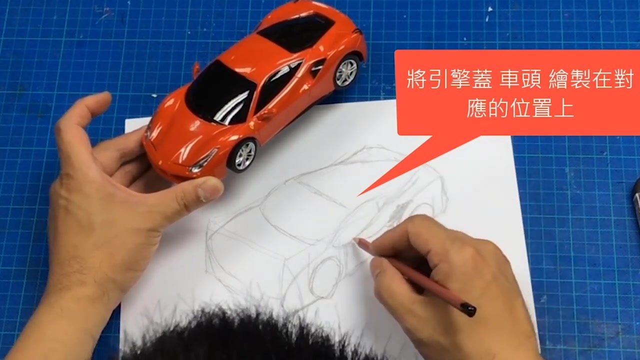 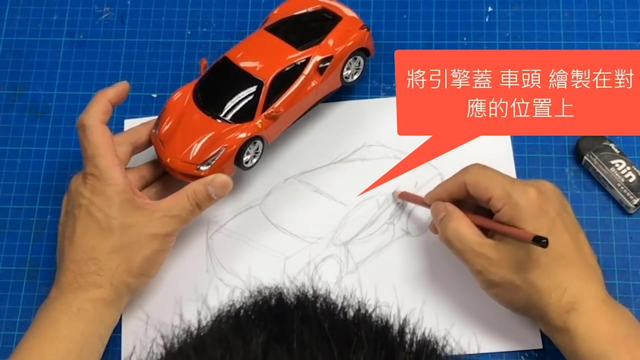 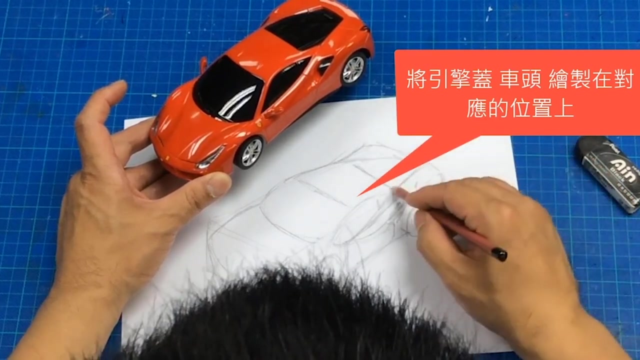 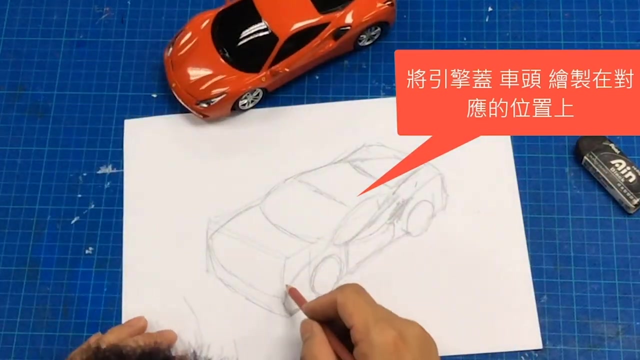 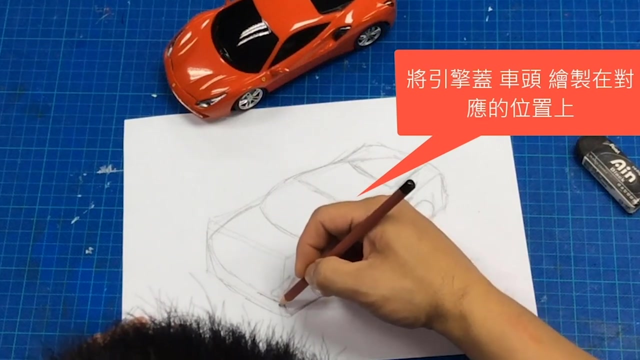 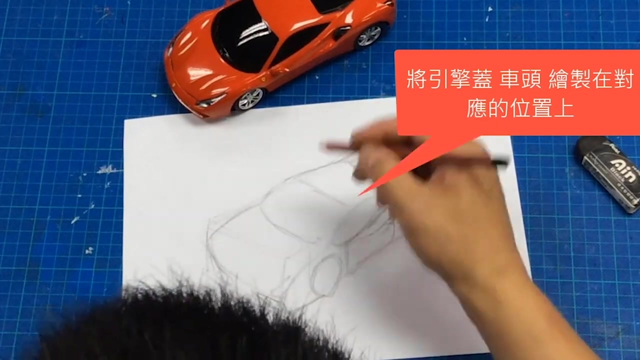 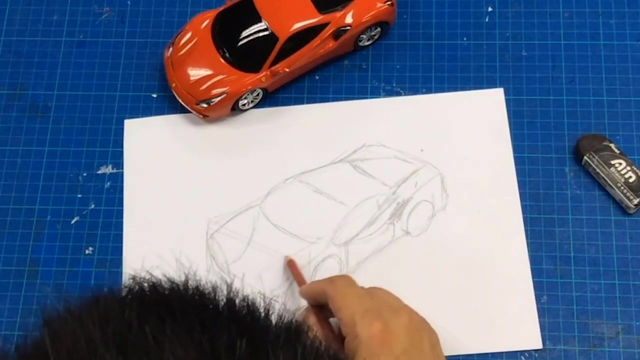 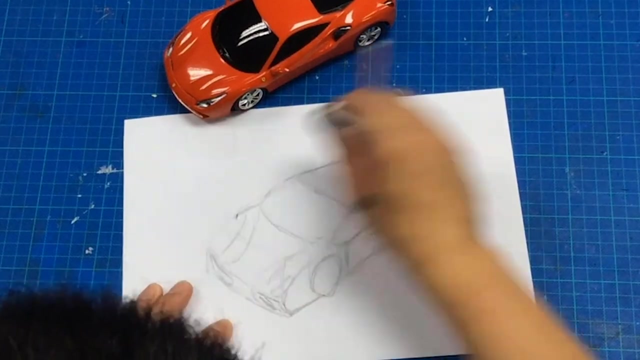 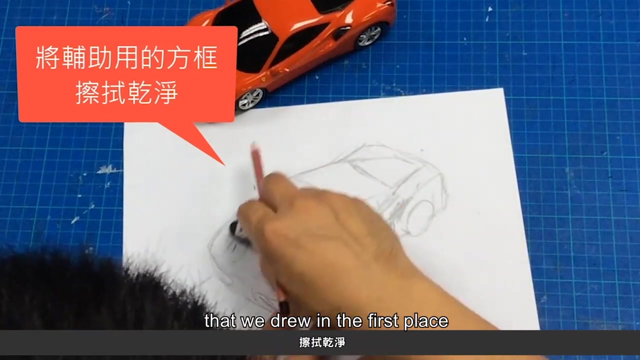 Finally, we draw the contour lines corresponding to the hood, the bumper and headlights in front of the vehicle. vehicle, Thank you, Thank you. Afterwards we have to erase the cube that we drew in the first place so that the contour features of the model can be highlighted. 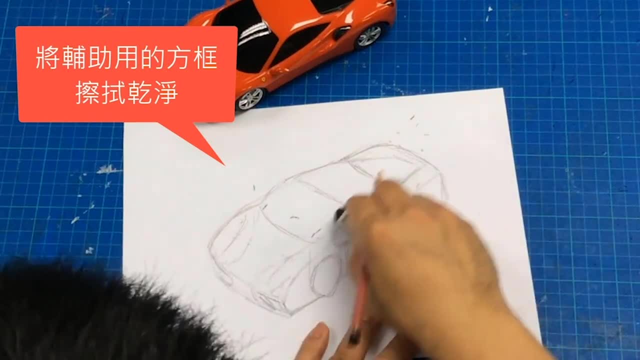 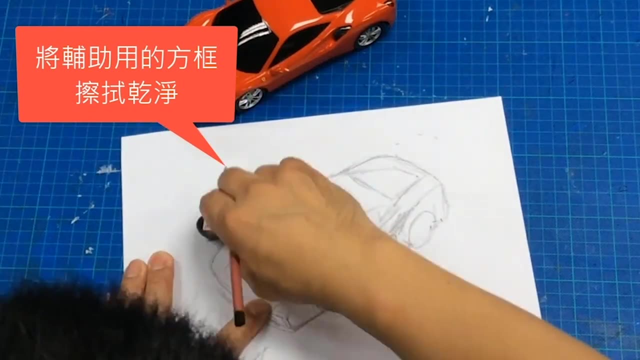 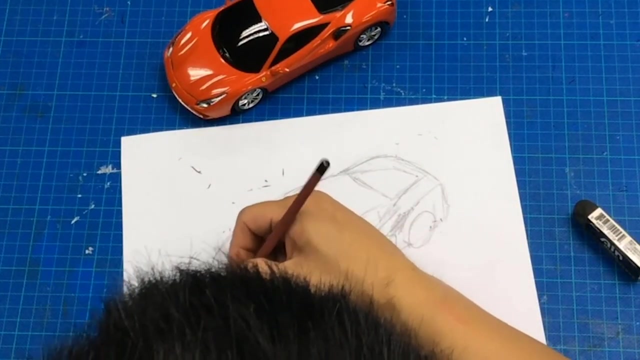 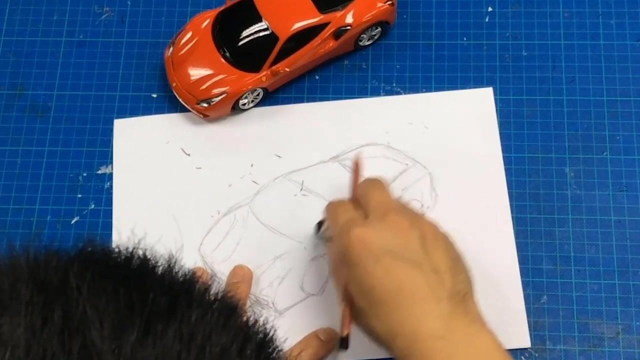 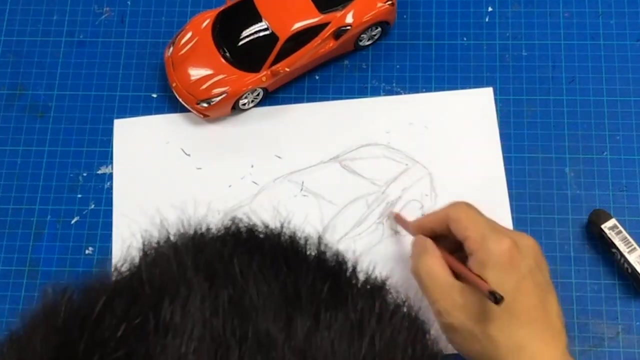 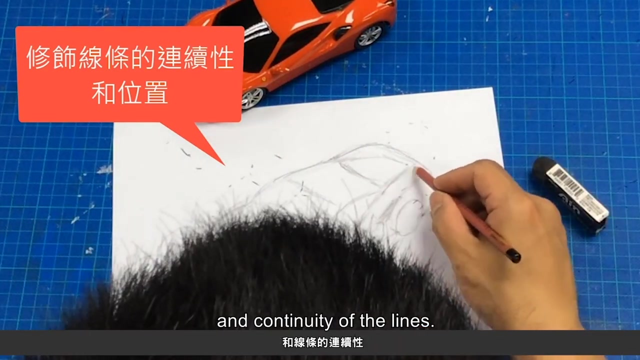 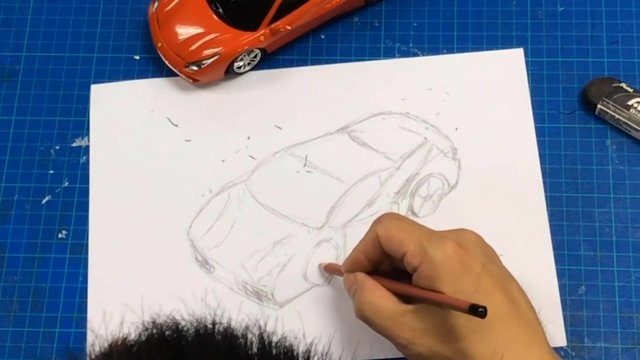 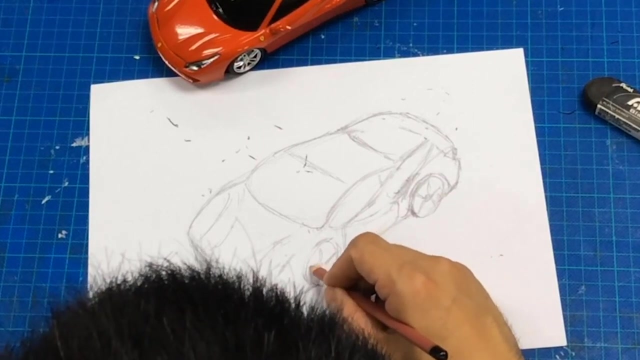 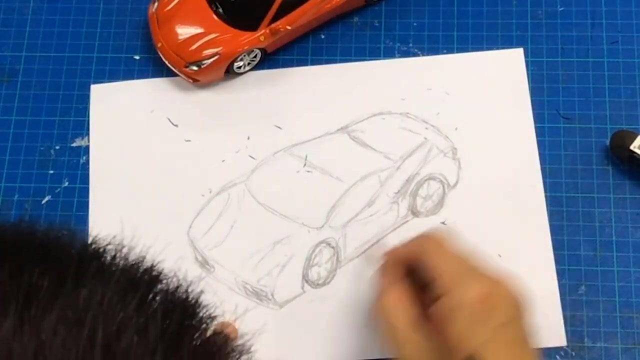 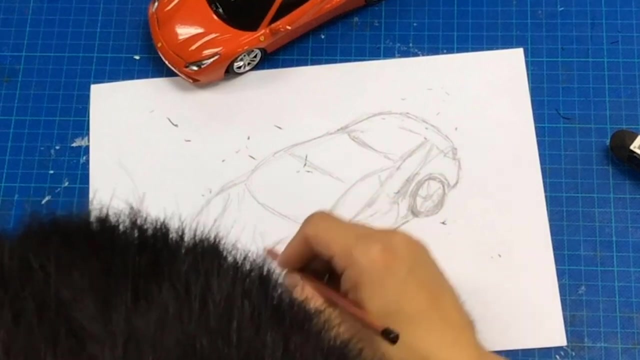 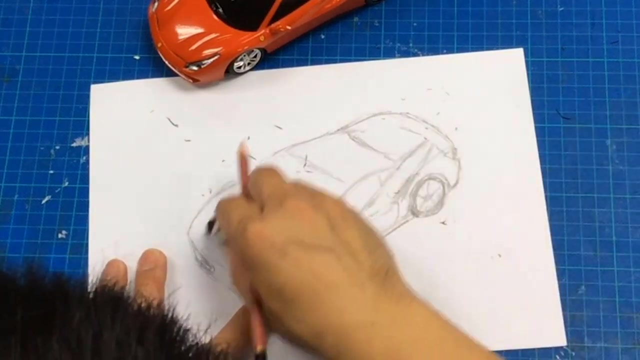 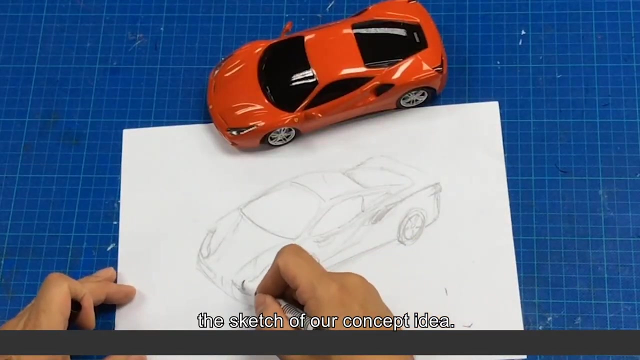 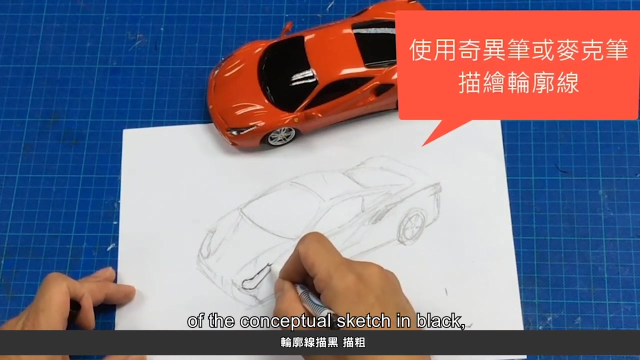 Thank you. Finally, we retouch the position and continuity of the lines. This way, we have completed the sketch of our concept idea. Next, I will demonstrate how to use a marker to outline the contour of the features of the conceptual sketch in black. 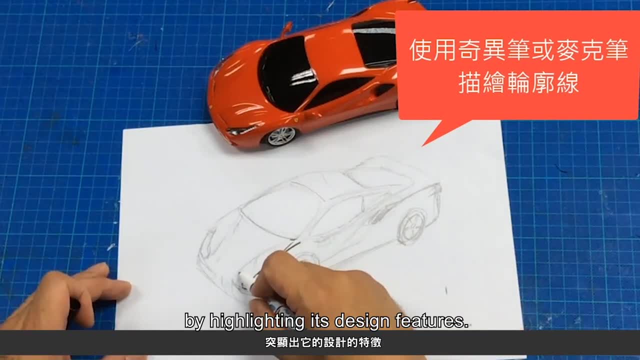 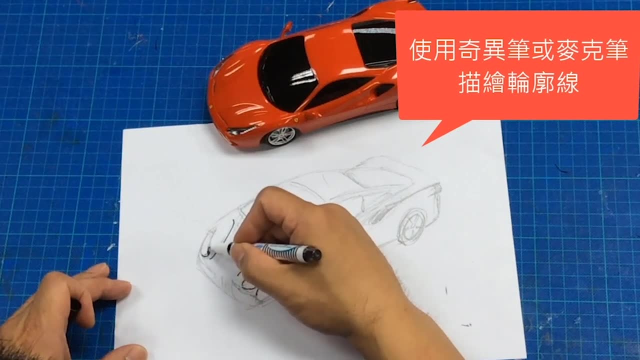 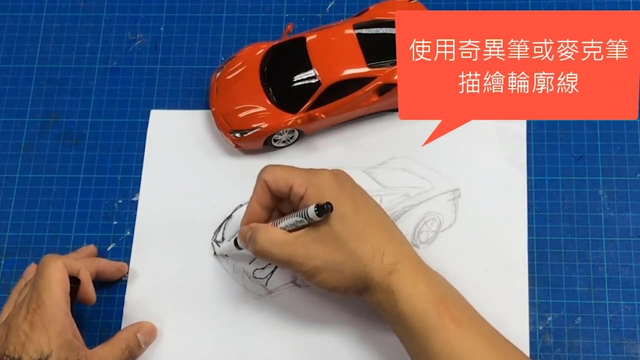 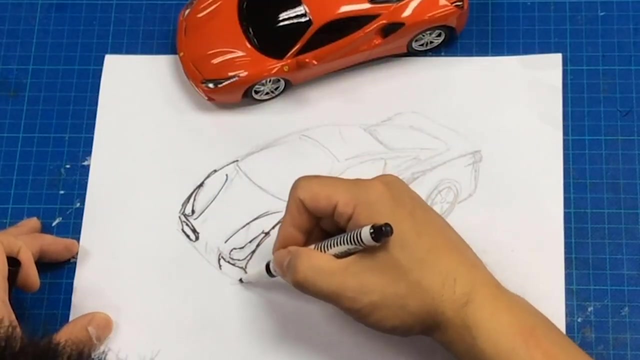 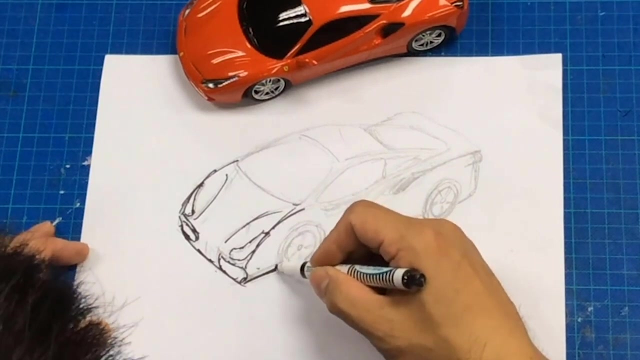 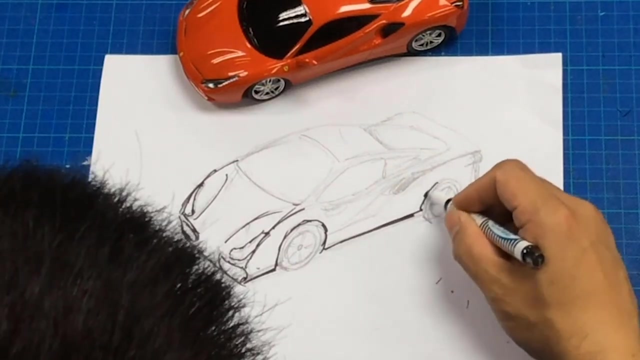 so that the model can be highlighted. Make sure that the sketch of the design has a more three-dimensional sense by highlighting its design features. The design features can be highlighted with a black pencil. The sketch is drawn with a black pencil. Now we will use the marker to highlight the contour. 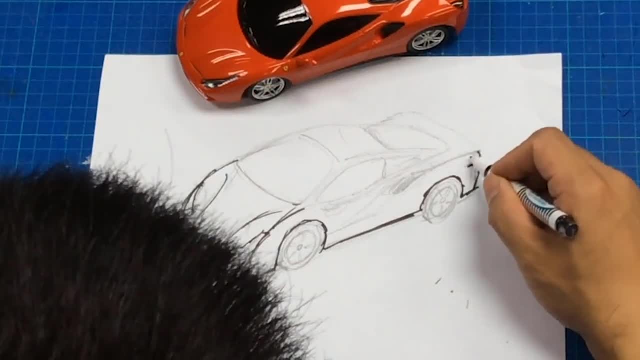 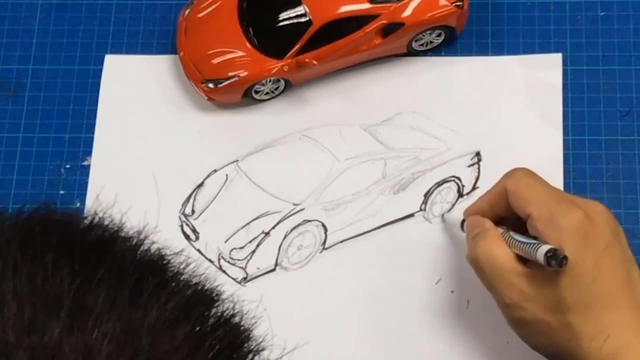 We are going to highlight the contour of the lines. First, we draw the lines separated toward the center of the model. The proportion of the lines is the same as the length of the line In the middle. we will draw the decal with the marker. 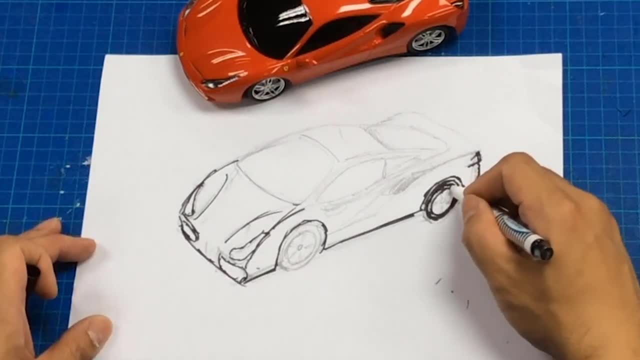 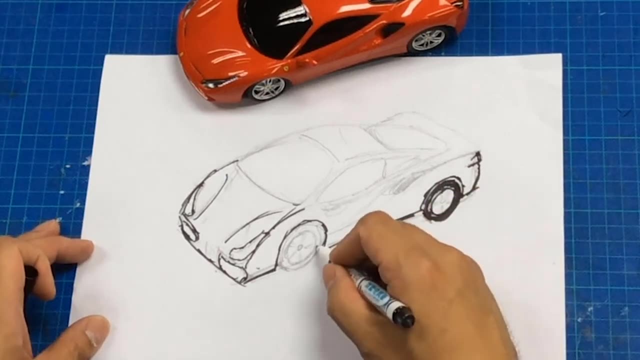 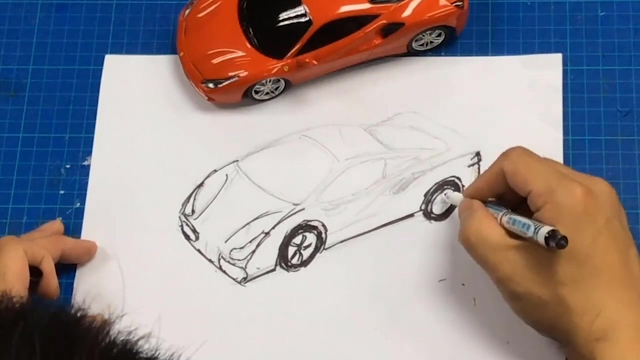 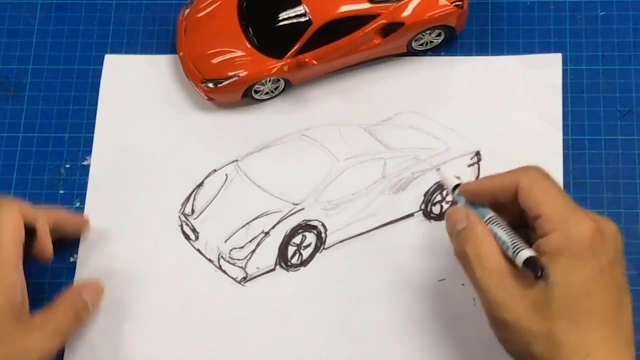 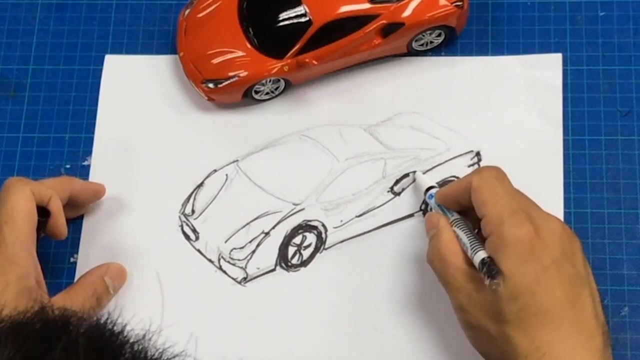 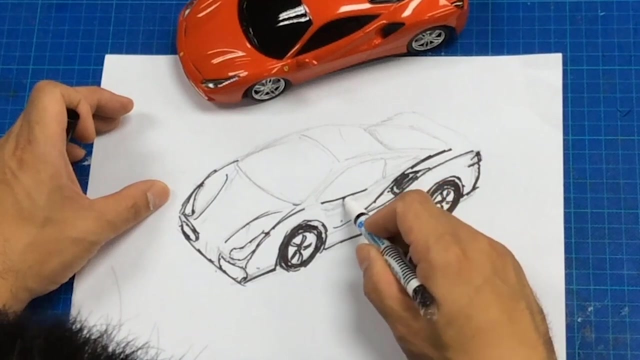 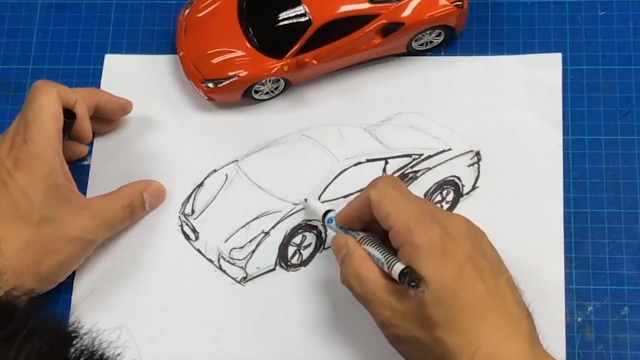 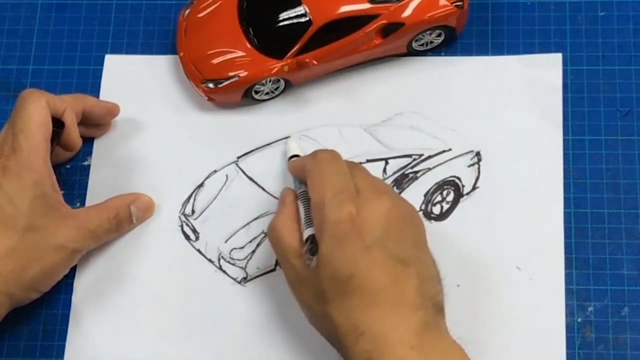 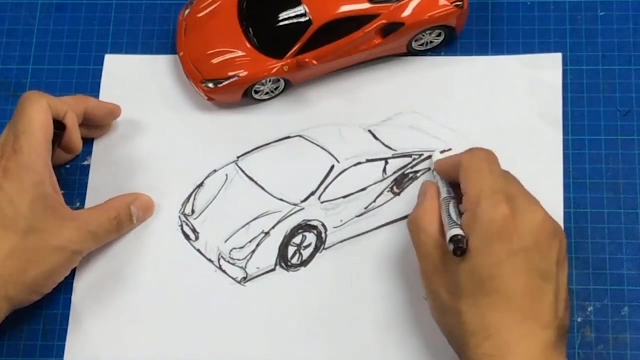 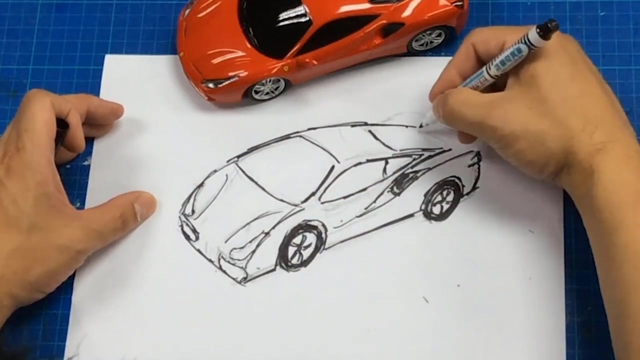 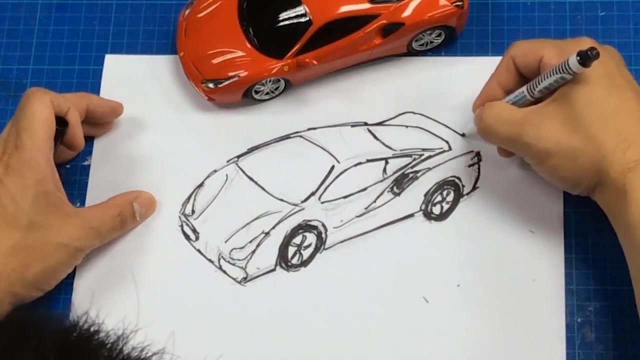 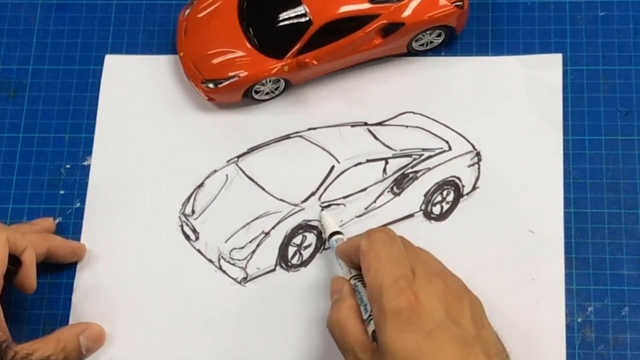 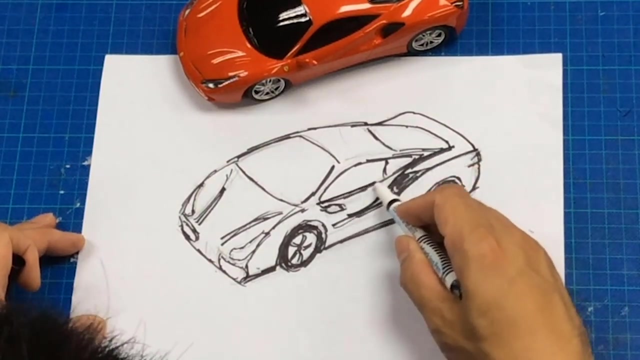 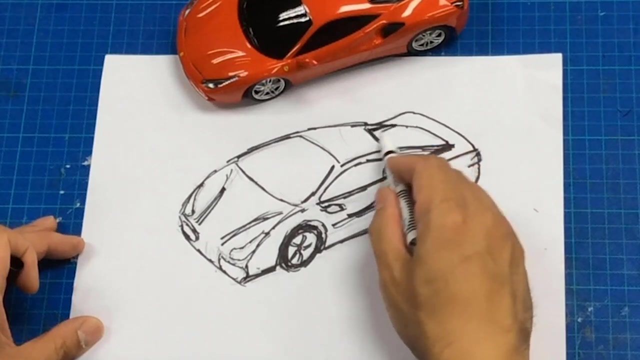 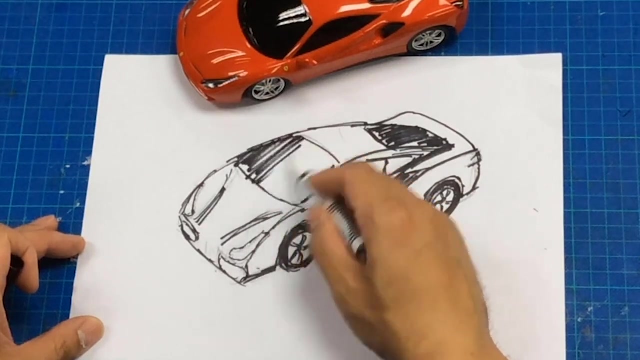 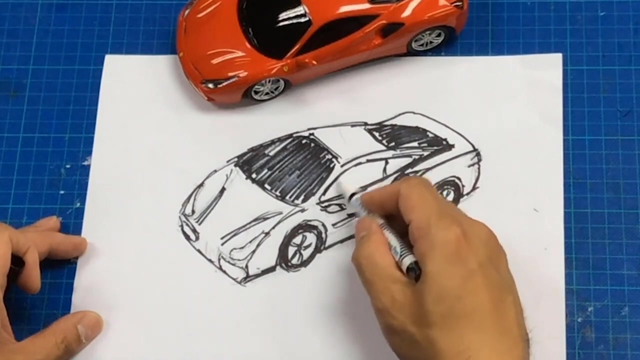 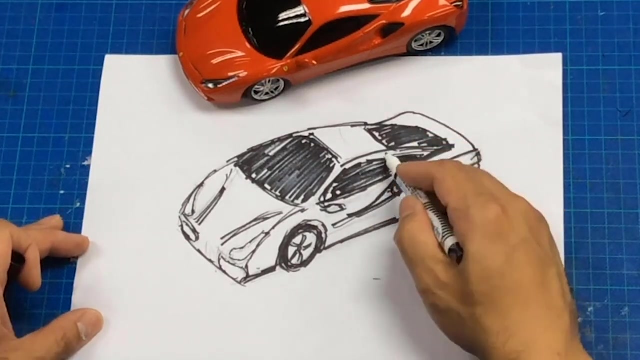 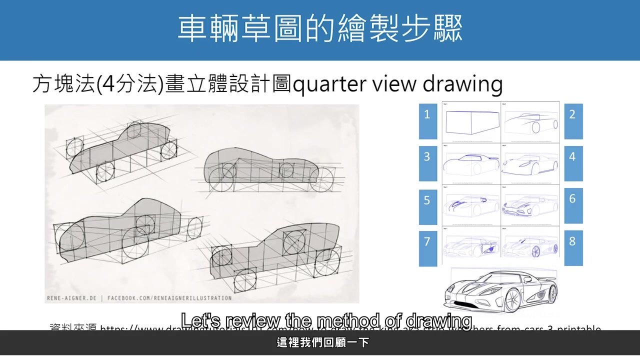 This is one example. Next, we will highlight the line: you, you, you, you, you. let's review the method of drawing the vehicle sketch that the teacher has just demonstrated. we use the cube method to draw the three-dimensional sketch, also called the quarter view drawing for. 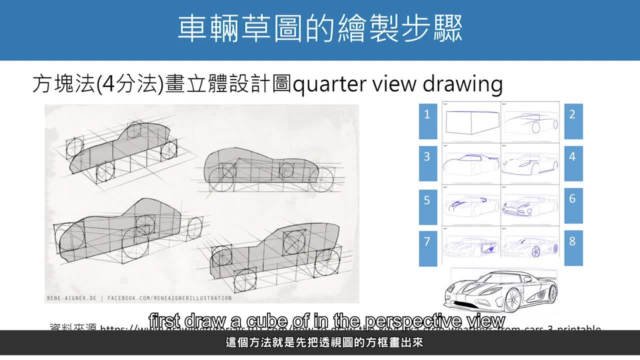 this method: first draw a cube off in the perspective view, then we use the wheel axles, as the corresponding position of the car body, to draw the contour line of the side of the car, as well as the top of the car and the front of the car, according to its corresponding relationship. 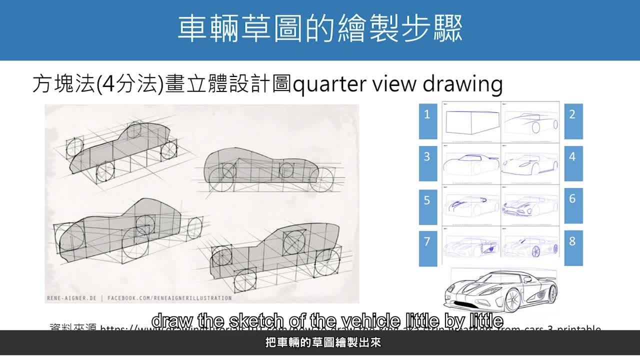 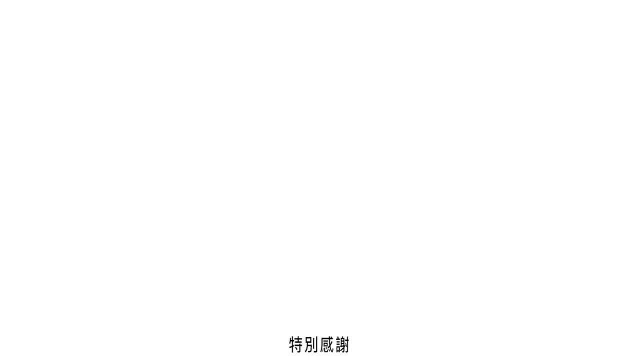 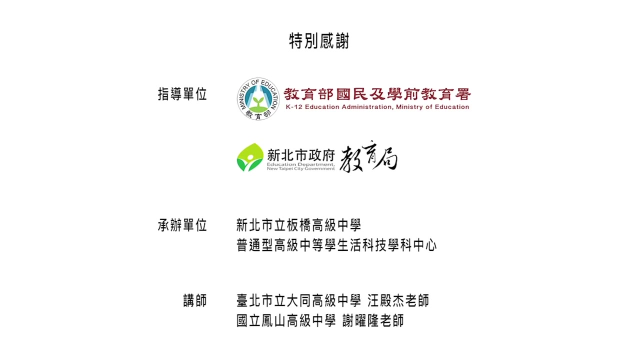 with this cube. draw the sketch of the vehicle little by little to its corresponding position within the cube. please take out a piece of white paper and see if you can draw a sketch of your idea. please feel free to leave the comment with comments below if you think this was useful. if you prefer this video, please like the video and subscribe to the channel and surely give a thumbs up. if you like the video, please press the bell icon and that way you will get notifications for future videos. thank you for watching. this video was very following and I hope you still. enjoy it. 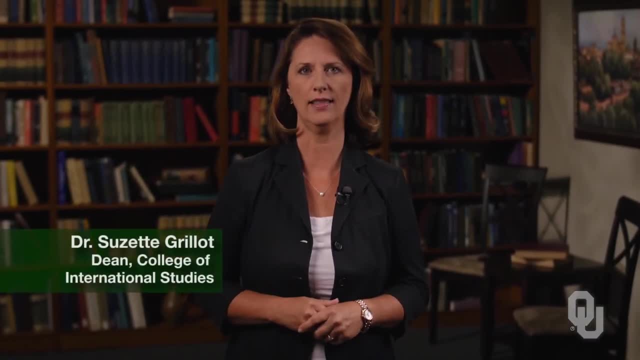 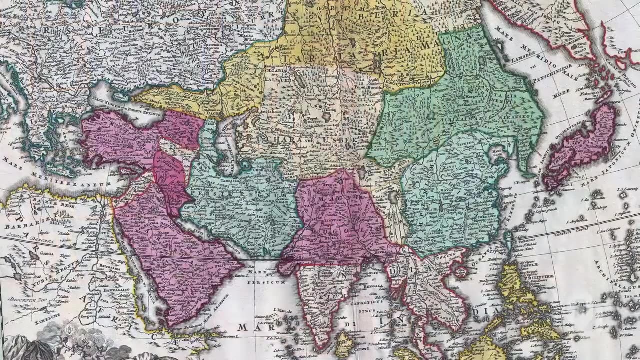 There are a number of academic disciplines that are useful in helping us understand the global community. One discipline that we will look at in this section of the course is geography. Broadly speaking, geography is the study of planet Earth's lands, features, inhabitants. 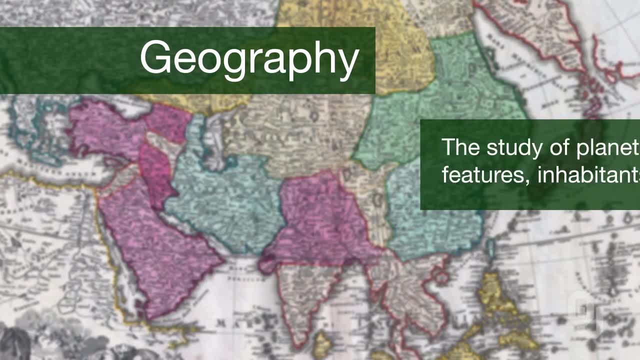 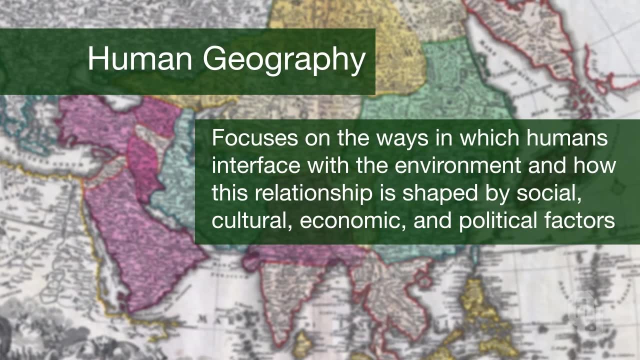 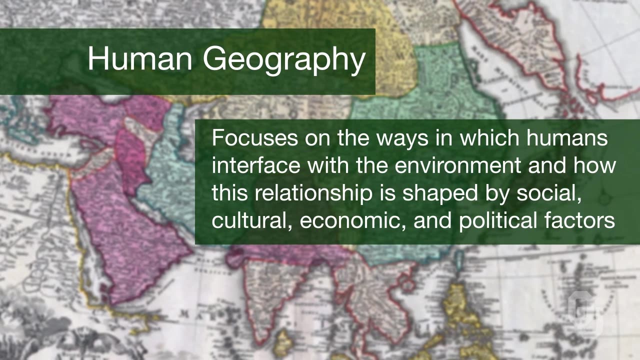 and phenomena. Geography is divided into two subfields, including physical geography and human geography. Human geography focuses on the ways in which humans interface with the environment and how this relationship is shaped by social, cultural, economic and political factors. Physical geography, which we will discuss here, is the study of planet 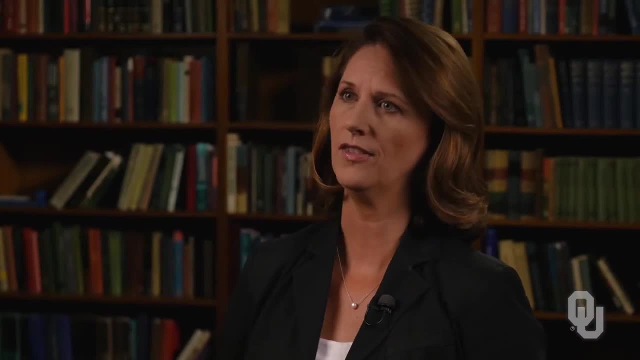 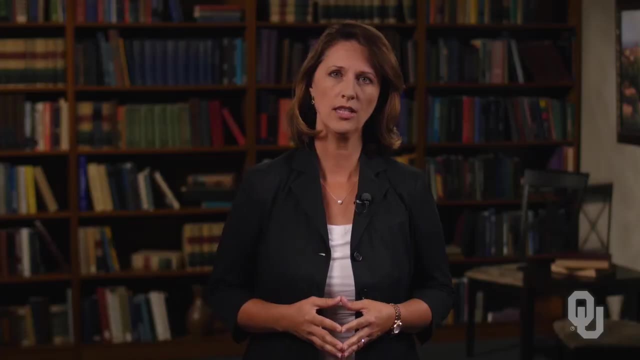 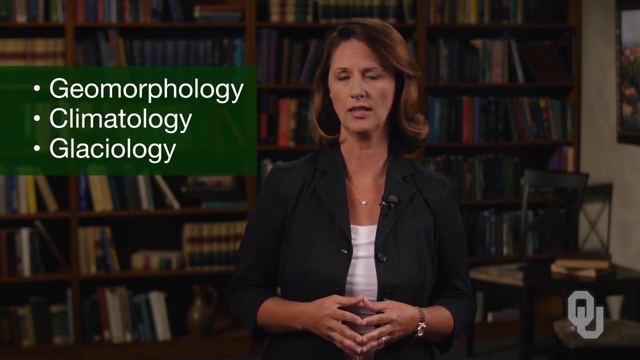 Earth, its resources and processes. The discipline of physical geography examines a wide range of the Earth's resources, from fossil fuels to gemstones to water. Additionally, physical geography explores the Earth's processes by drawing on other fields of study, such as geomorphology, climatology and geology. 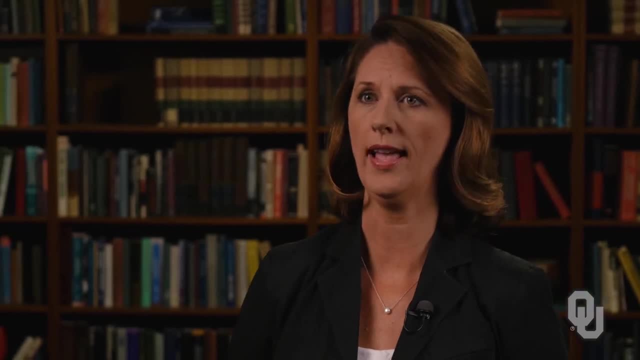 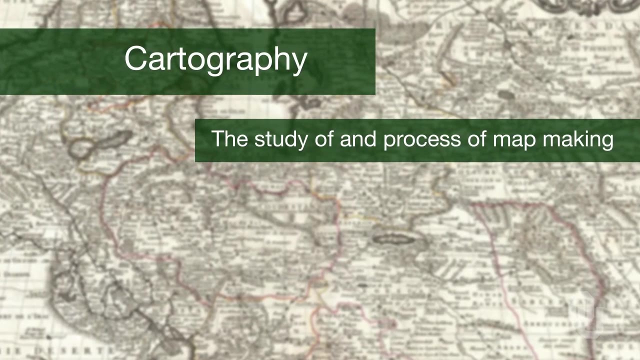 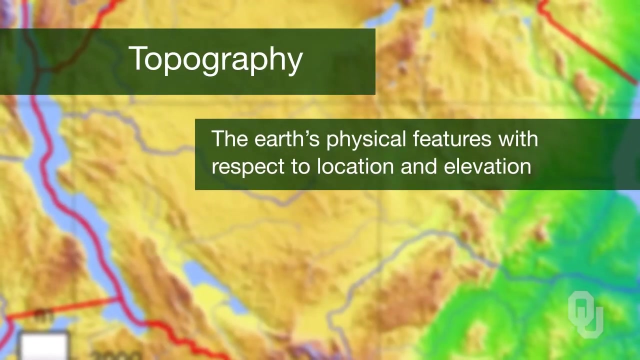 Cartography is one very important way in which we conceptualize both physical geography and human geography. Cartography is the study and process of map making. Maps are used to depict many aspects of physical and human geography. Maps can show topography, which are the Earth's physical features with respect to location and elevation. These features 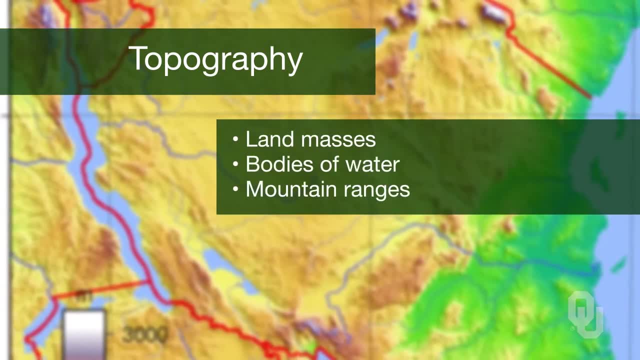 can include things like land masses, bodies of water and mountain ranges. Maps can also depict things like physical borders, land masses and mountain ranges. Maps can also depict things like land masses, bodies of water and mountain ranges. Maps can also.